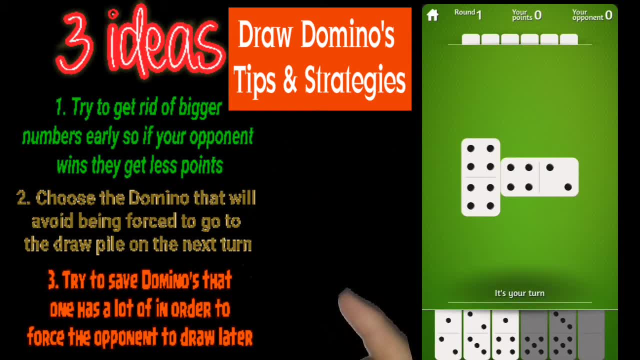 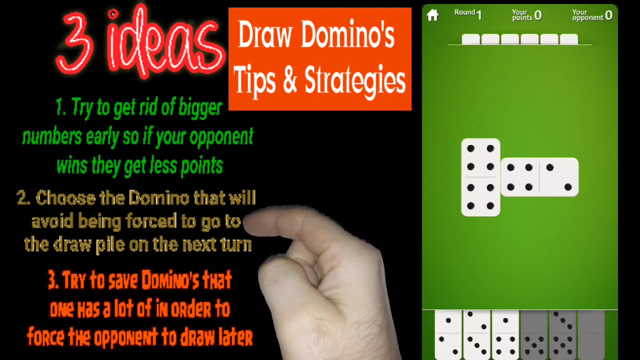 on the next turn. Now, the second tip that I have here is that you want to try to make it so that you're going to be guaranteed a turn on the next turn. So there's a 2 and a 4.. What we're going to want to do is probably either play the 2-1 over here or alternatively. 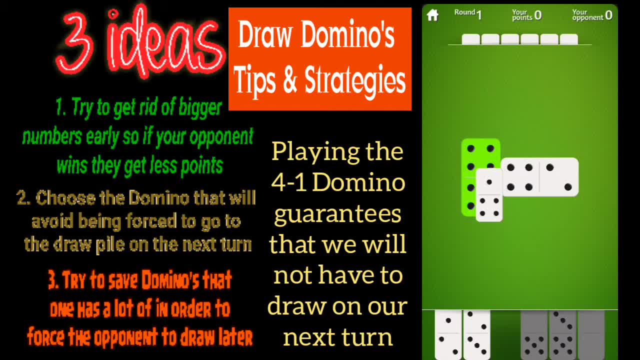 we could play the 4-1 on this side. Since the 4-1 is worth more points, we're going to take that one and get rid of that. That's going to guarantee that, no matter what our opponent does, we'll be able to move on. 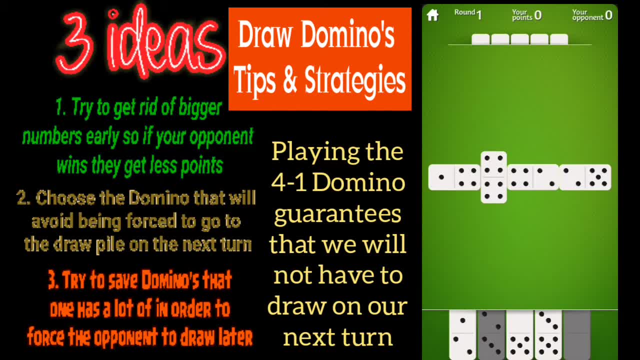 At least one domino on the next turn, And then we would follow through to that. So in this case, we have a 1 and a 2.. We have a 5-0 and a 5-3.. We could either play the 5-3, which will allow us to. 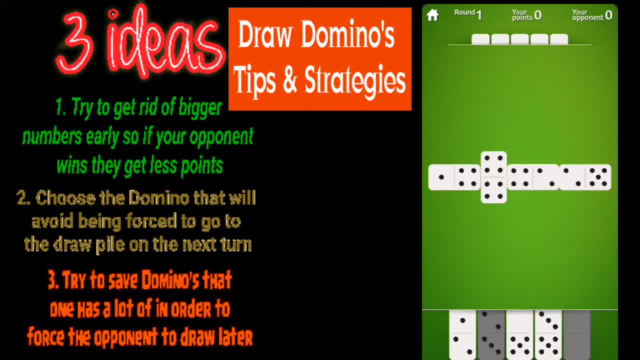 play the 3-2 next turn, or we could play the 5-0.. I would prefer the 5-0 in this case because we want to get rid of that double zero, Even though it's not worth any points we could be stuck with. 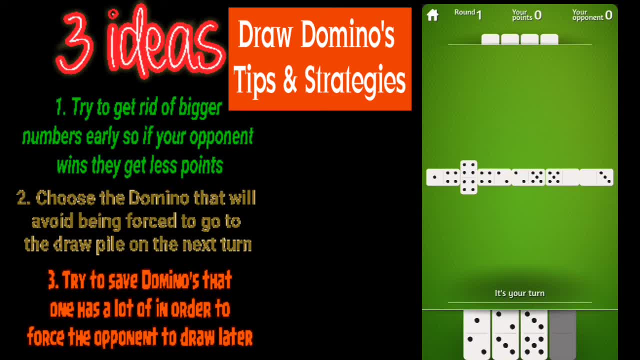 it later on, And there our opponent plays that. So now we have a choice between the 3-5 and the 3-2.. I'm going to go ahead and play the 3-2. So we're guaranteed a move on the next turn, Although you can make a. 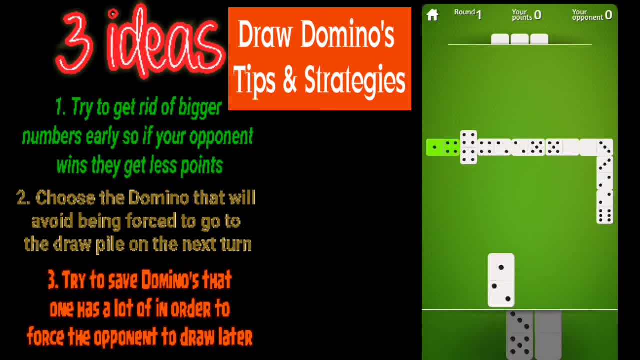 case for the 5.. But you typically want to have moves or be able to make moves. Otherwise you're going to be forced to go to the draw pile. Here we get lucky. They played that. Now we're just left with a double zero. That's not worth a lot of points And our opponent is forced to draw Of. 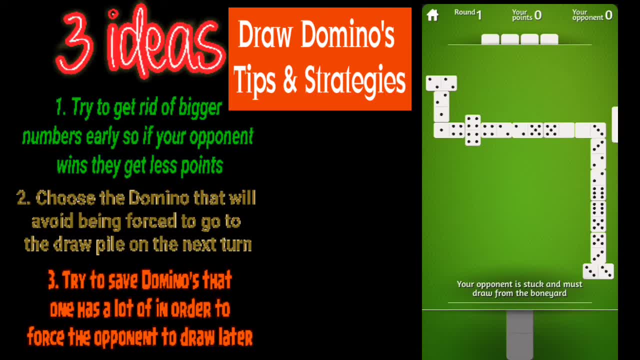 course, we're going to be forced to draw there, But that's the general idea, Is that you want to set up your opponent, get them to draw and try to give yourself options. In this case, we're going to be drawing, But we're in pretty good shape. Now we get the zero out there, I think. 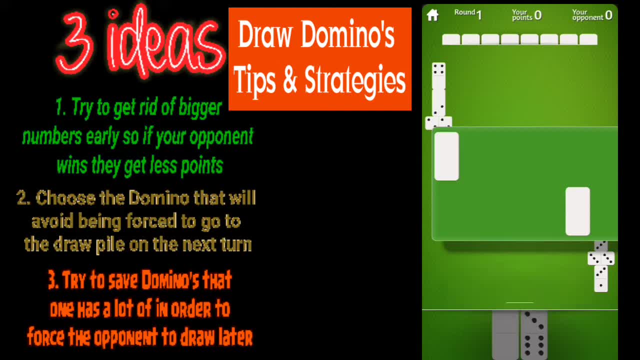 our opponent has a zero as well. But again, even if we lose on points here, we're not going to lose on points if it comes to a draw. In this case, we get rid of the 6 and the 3.. We've got no points left. 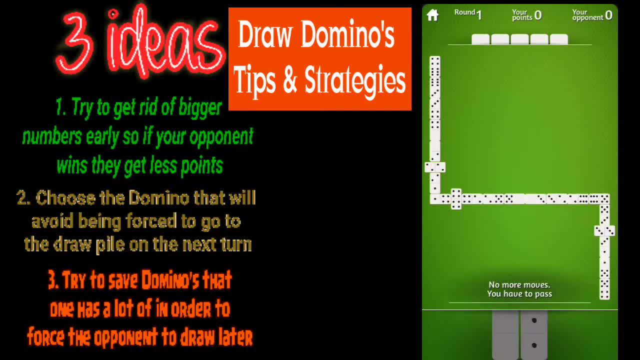 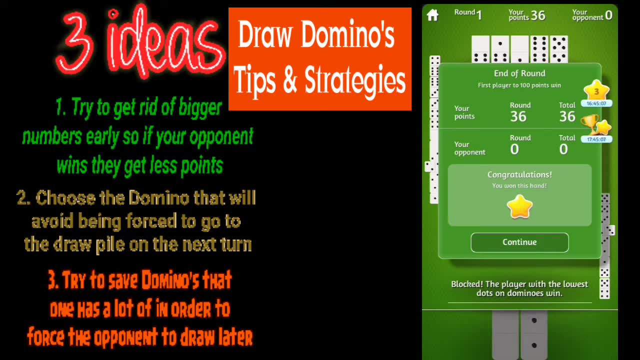 So even if our opponent runs out, it's going to end up being a draw on the round. In the worst case scenario now we would give up two points And it came down to a showdown. We got 36 points right there.